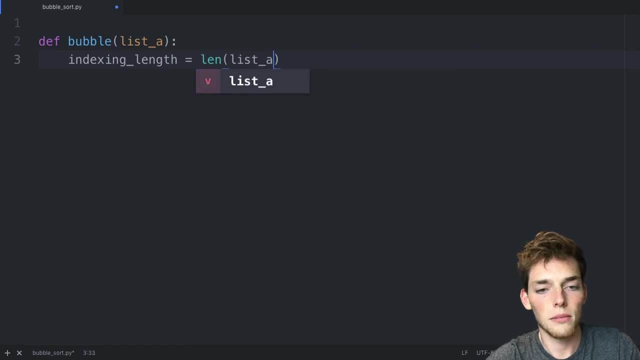 and this will be equal to the length of list A minus one. We're saying minus one here because we can't perform a comparison on the last number of the list because there's not a number after it. So we'll do this up to the minus one element. Now we'll drop down, We'll create. 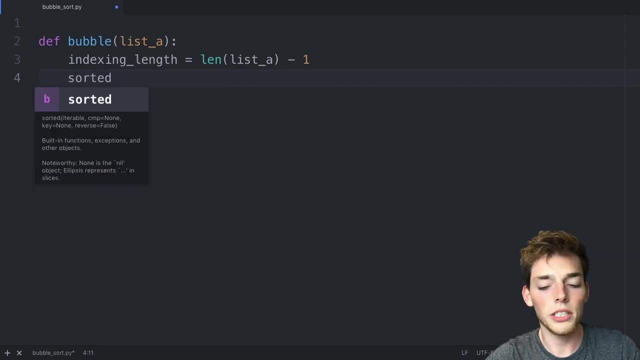 a local variable that we'll use throughout this function. So we'll say: sorted is equal to false. We'll use this sorted variable inside our control flow to break us out whenever the list has been sorted. Now we'll drop down, and we need to perform this at a number of iterations that we don't know. So to do that, we'll say: 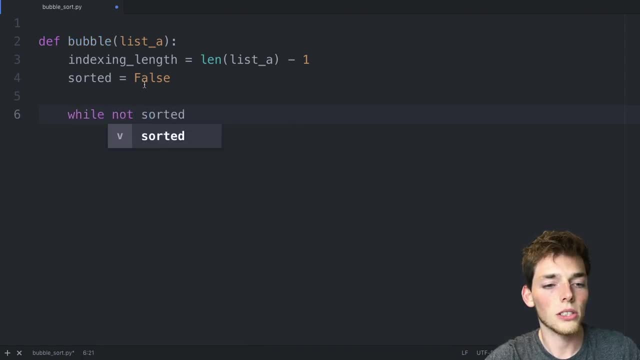 a while loop and we'll say while not sorted. So as long as this variable is false, we'll do these actions. Now we'll reference that local variable again. We'll say sorted is equal to true. This line of code here will make sense in just a second. We'll drop down. 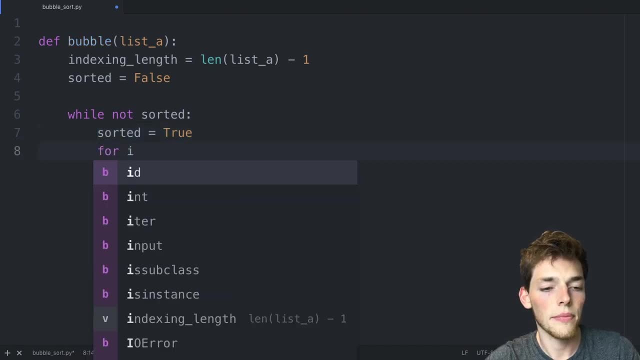 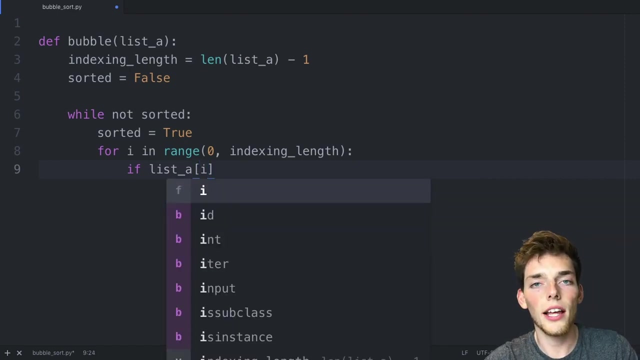 and create a for loop. So we'll say for I in Then range of zero to our indexing length. We want to do a comparison. So we'll say if list A in the I position- so this will be the value to the left- is greater than the, 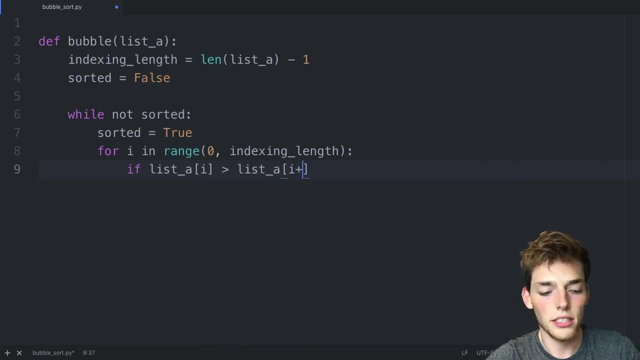 value at list A in the position to the right. So I plus one. We need to say sorted is equal to false, And then we need to flip those two values in our list. We can do that by saying list A indexed at the I position and then list A- I plus one, is equal to the opposite. 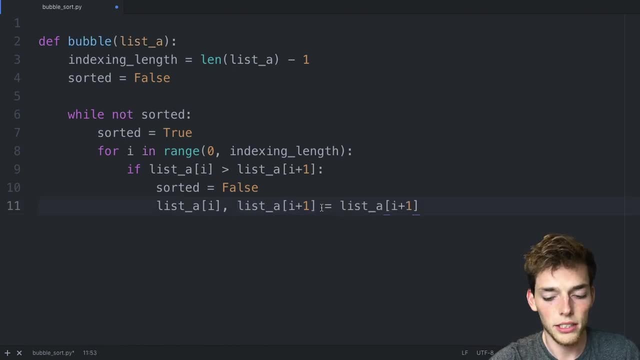 So we'll put this value first, We'll copy it and paste it here, And then we'll put this value second. Copy that and paste it here. So what we're telling our algorithm to do is that if an item in the list to the left is greater than the item to its right, then 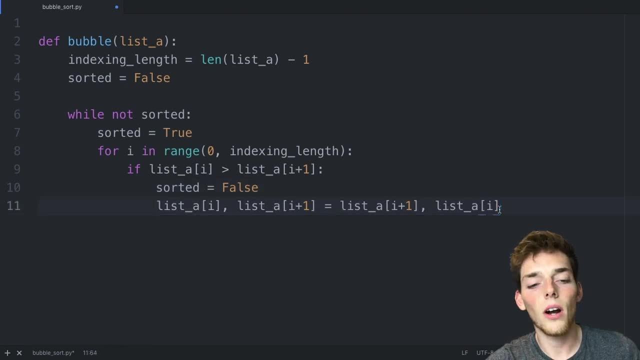 it needs to be sorted if it's a buttered item. So we can just sort all of our items and this if statement here will take back its value and we'll leave the ill- 74% of the Kh and possibly flip those two items. Whenever we've sorted all of the items, this 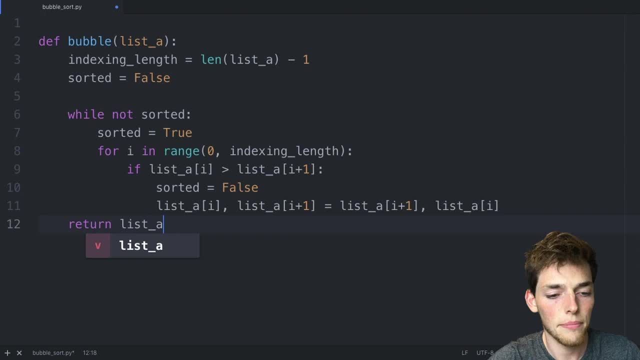 if statement won't activate, so the sorted variable will just remain true and that will break us out of this while loop. Finally, we just need to return the now sorted list. We'll drop out and then back over And we'll say: return list A.